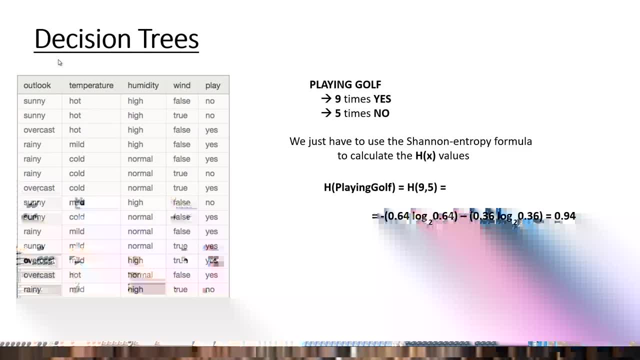 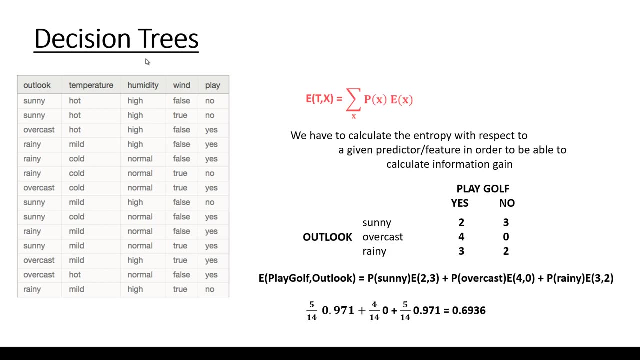 In the previous lecture, we have been talking about how to calculate Shannon entropy for a given feature. Of course, we are interested in the target variable, so that's why we have to deal with the Shannon entropy of playing golf. Okay then we have to calculate the entropy with respect to a given feature. As far as 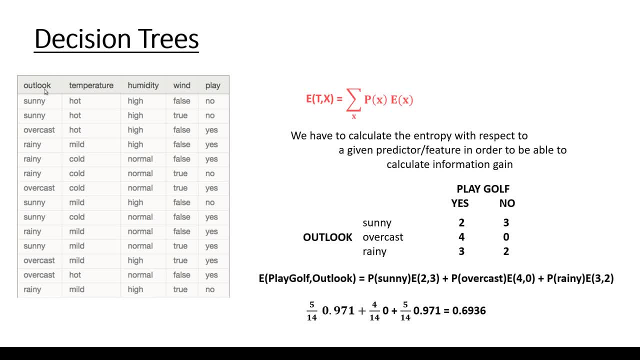 the dataset is concerned, as you can see, we have 4 features- outlook, temperature, humidity and wind- and we have a so called target variable- whether we are going to play golf or we are not going to play golf. So this is the formula we have to use. We have to find out the probability. 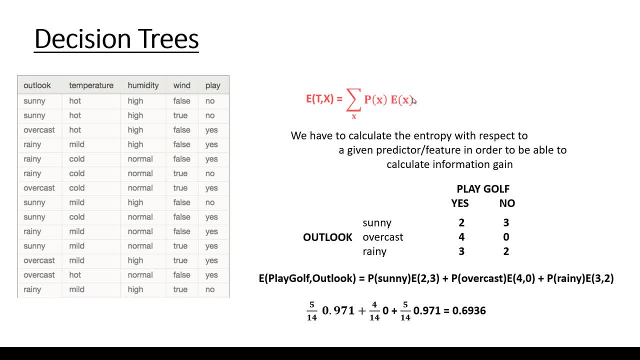 of the given feature, we have to multiply it by the entropy and finally, we have to sum them up. Let's take a look at the outlook feature. As you can see, there are three possible values of the outlook. The outlook can be sunny, it can be over-costed and it can be rainy. 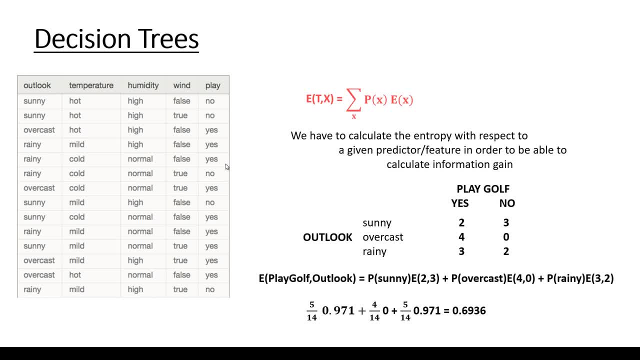 So this is why we have sunny, over-cost and rainy, And we have the target variable, whether we are going to play golf or not. So, basically, there are two possible values of playing golf- yes and no, And we just have to count the occurrences. 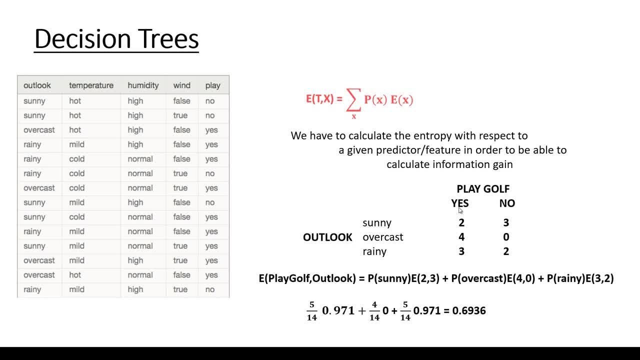 So, for example, whenever the outlook is sunny, how many yes and no values are there in the play column? So sunny has the value no, sunny has the value no. then sunny has the value no, then sunny has the value yes. and finally, sunny has the value yes, which means that there are two. 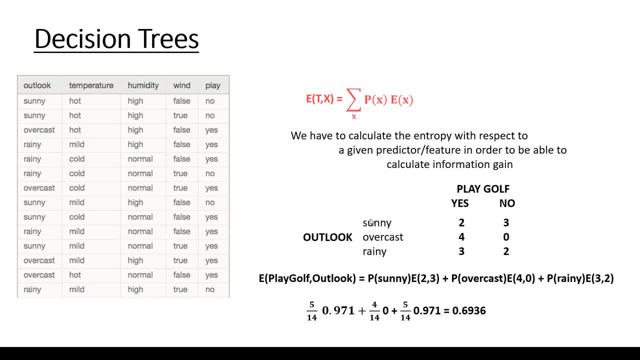 yes values and three no values associated with sunny. We have to do the same for over-cost, and we came to the conclusion that we have four yes values and zero no values. What about rainy? We have three yes values and two no values, So we just have to use this formula. 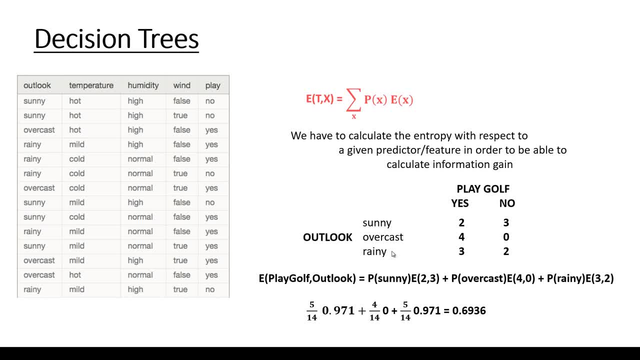 We have to calculate the probability of the given possible values. What is the probability of sunny? We have 1,, 2,, 3,, 4,, 5,, 6,, 7,, 8,, 9,, 10,, 11,, 12,, 13, 14 values all together. 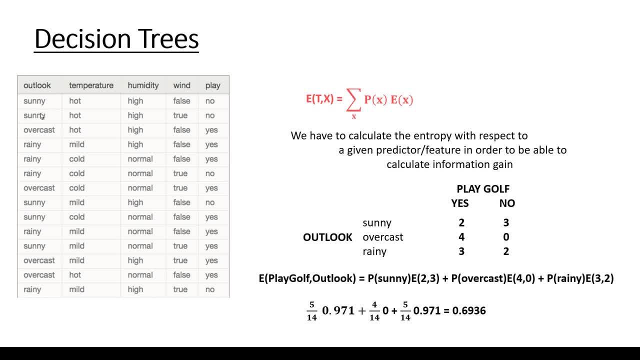 And we have to count the occurrence of the sunny, So we have 1,, 2,, 3,, 4 and 5.. So this is why the probability of sunny, as far as the outlook feature is concerned, is 5 divided by 14, and we have to calculate the entropy with these values: 2 and 3.. 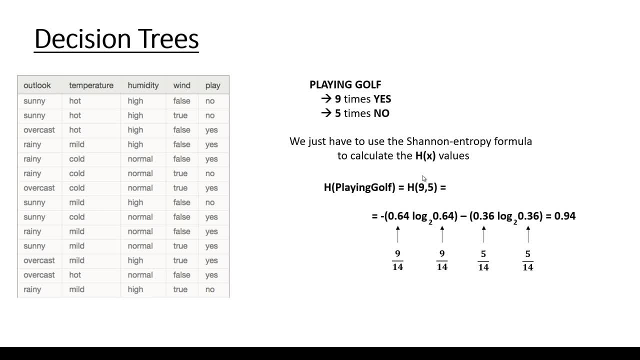 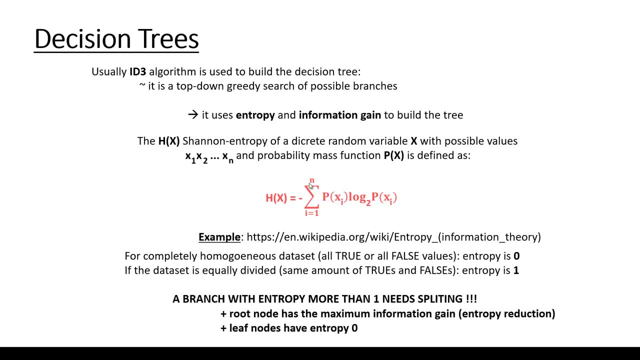 This is what we have been talking about in the previous lecture, that calculating this entropy we just have to use this simple formula. This is called the Shannon entropy, So the probability times the base 2 logarithm of the probability. We take the base 2 logarithm of the probability and we have to calculate the entropy over. 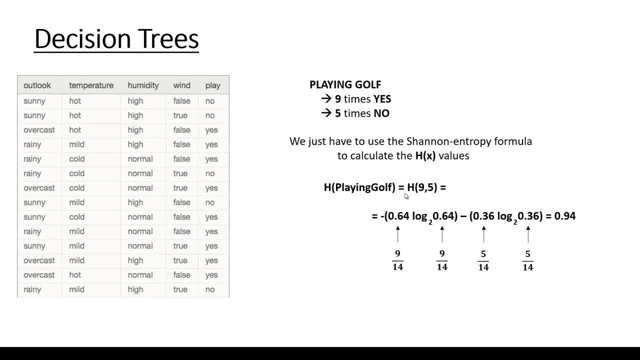 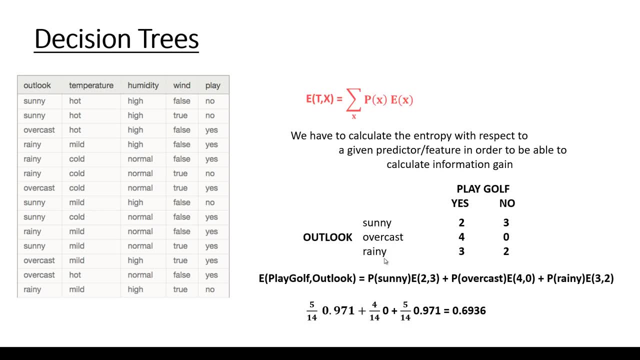 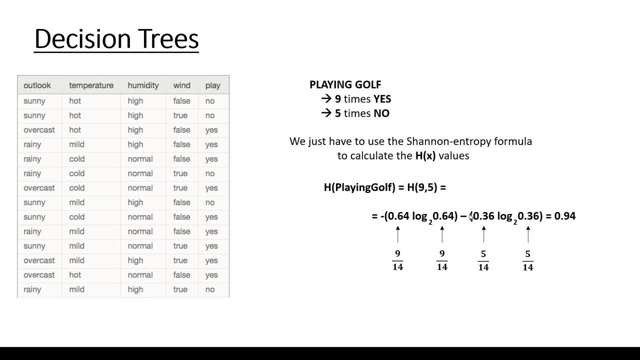 two- the probability- and we have to sum them up. so in this case, for 9 and 5, we have something like this: whenever we have 2 and 3, what do we have to do? we have to use 2 divided by 5 base 2, logarithm: 2 divided by 5 minus 3 divided by 5 base 2. 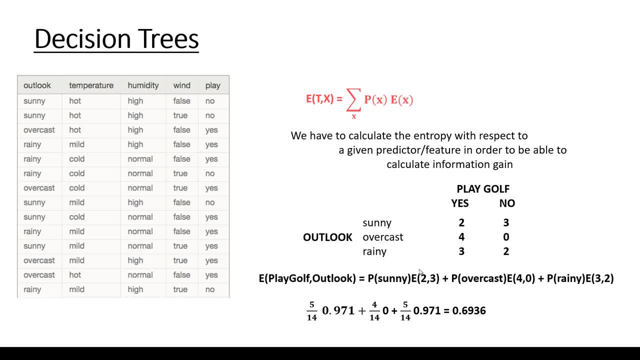 logarithm 3 divided by 5. so we have to use the same formula as here, but of course with with these values, so 2 and 3, and it has a value 0.97 and 1. so basically, this is what we have to do. what is the probability of overcost we? 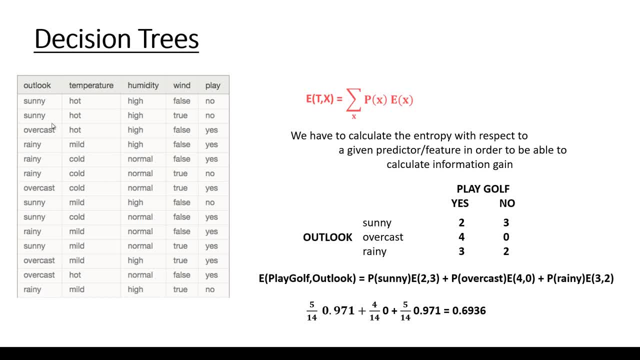 have 14 values all together and we have to count the occurrence of the over cost. so 1, 2, 3 & 4. so this is why 4 divided by 14 is the probability that the outlook is over costed. and what is the entropy? 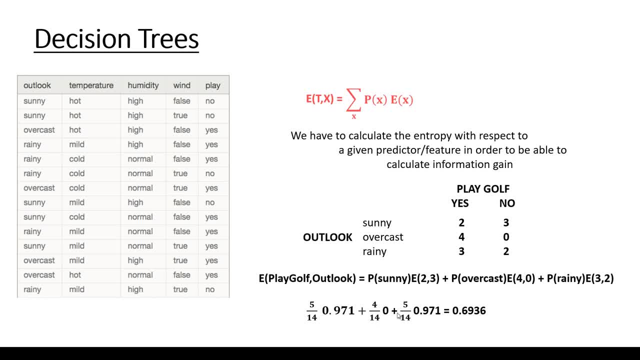 of value of our conclusion. for the value of our conclusion, for the value of the for four and zero, it's going to be zero plus the probability of rainy. how many rainy values are there in the outlook column? we have one, two, three, four and five. so that's why five divided by 14. 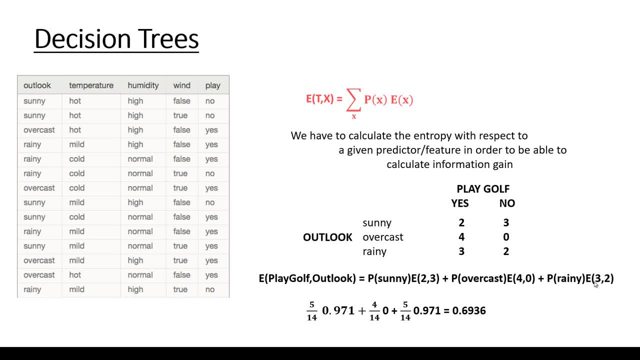 is the probability of rainy, and we have to calculate the entropy with three and two. again, we have to use this formula with the shannon entropy. by the way, if we sum up the probabilities, of course, we end up with one. so five divided by 14 plus four divided by 14 plus five divided by 14, 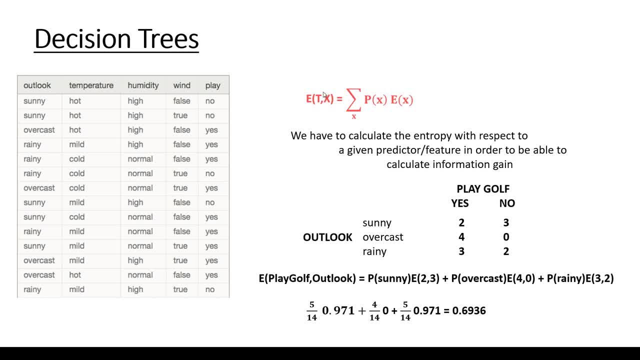 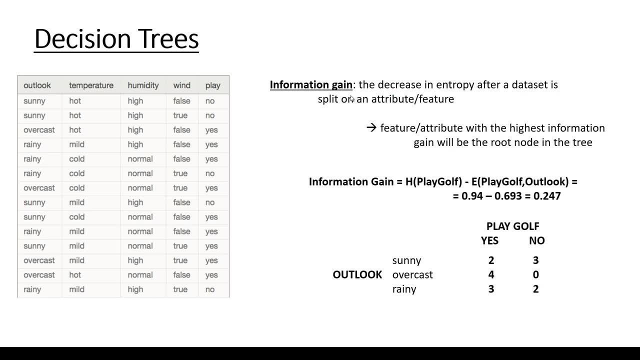 is equals to one, of course. okay, so this is how we calculate the entropy with respect to a given predictor or feature. and what about information gain? information gain is the most important value as far as decision trees are concerned. so, first of all, what is information gain? information gain- 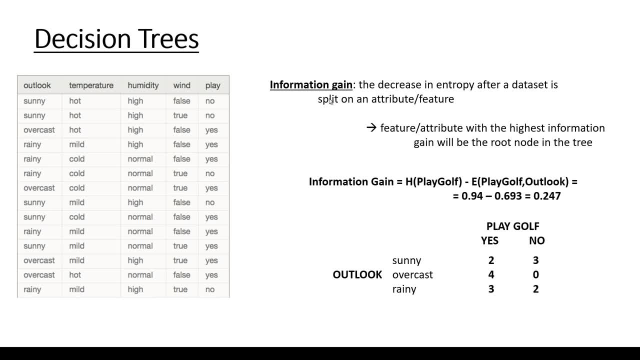 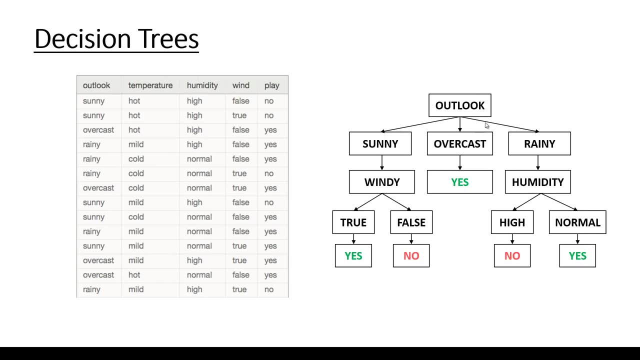 is the decrease in entropy. you the data set is split on a given attribute or feature feature, and attribute with the highest information gain will be the root node in the tree. in the previous lecture we have managed to construct the decision tree, but it is a good question that how do we decide what's going to? 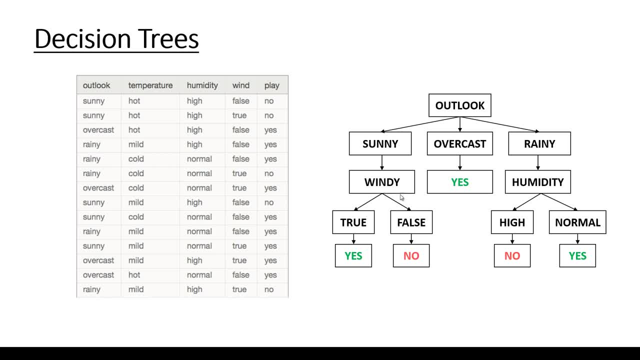 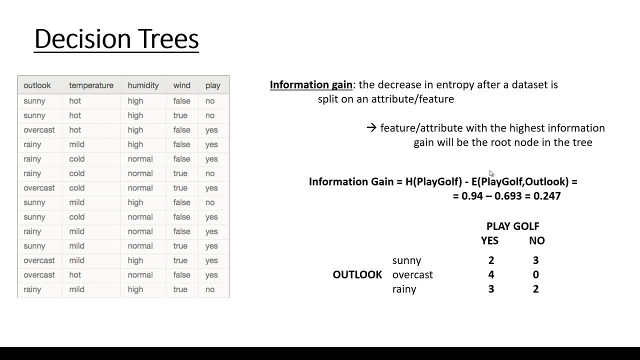 be the root node. how do we decide whether we have to split a given node or not? this is why we have to deal with information gain. so the information gain as far as outlook is concerned is the entropy of playing golf minus the entropy of playing golf with respect to outlook. so we have 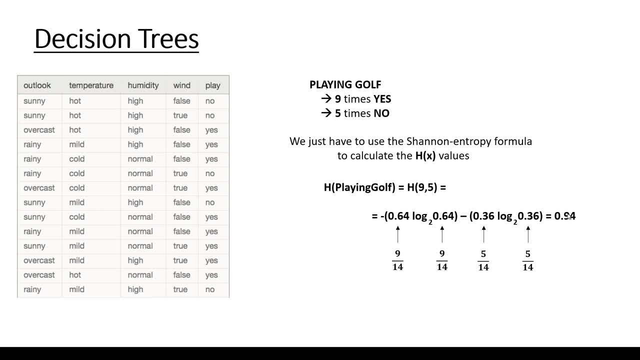 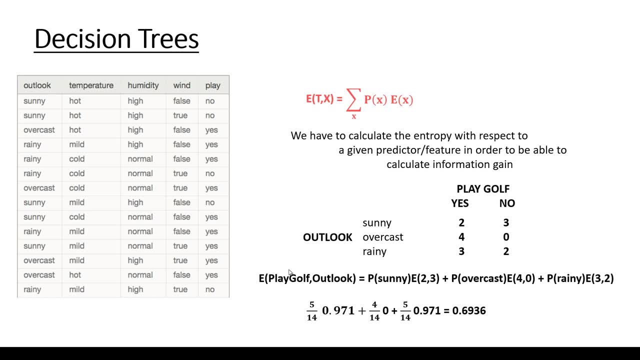 calculated the entropy of playing golf, which is 0.94. so this is why we have this value. and we have calculated the entropy of playing golf with respect to outlook, which is 0.69, 36, okay, so this is why we use this value and the result is going to be zero. that to see you in the next video. bye, bye. 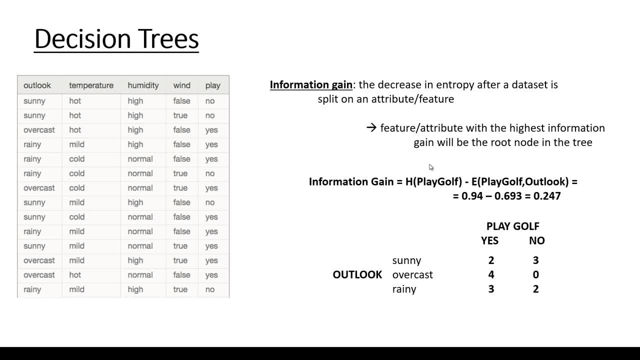 274.. So it is the information gain of playing golf with respect to Outlook, And this is what we have to do with all the features. So for Outlook, temperature, humidity and wind- And the feature with the highest information gain is going to be the root node in the tree. We just 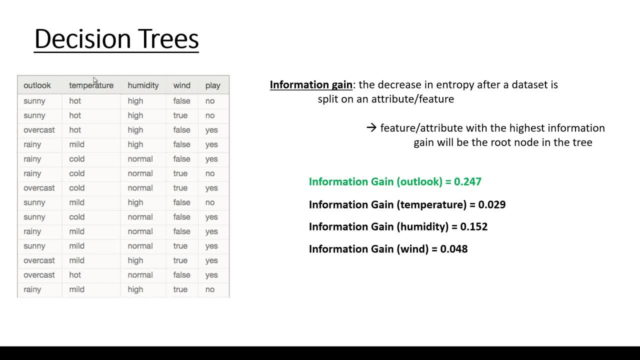 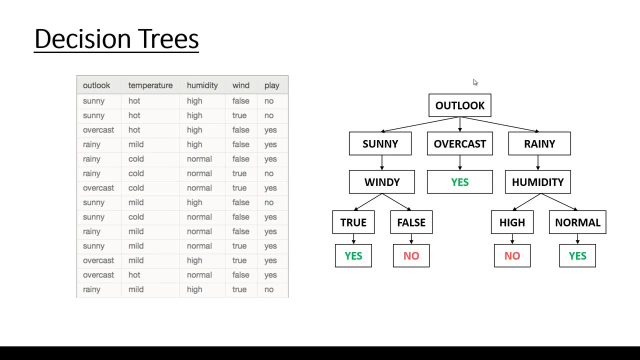 have to calculate this information gain for all the other features, such as temperature, humidity and wind, And we have to choose the one with the highest value. Why is it good? Because if we have the feature with the highest information gain, we know that it's going to be the root node in the 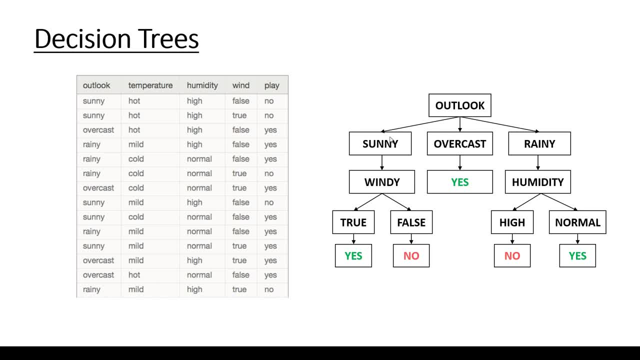 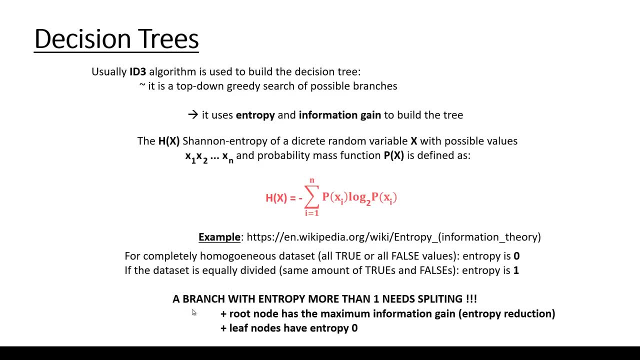 decision tree, because it is the most relevant feature. So this is how we are able to end up with an algorithm capable of constructing a decision tree. Okay, we just have to check that if an entropy for a given branch is greater than one, we have to split the given feature. So as far as overcost is concerned, we don't have to split. 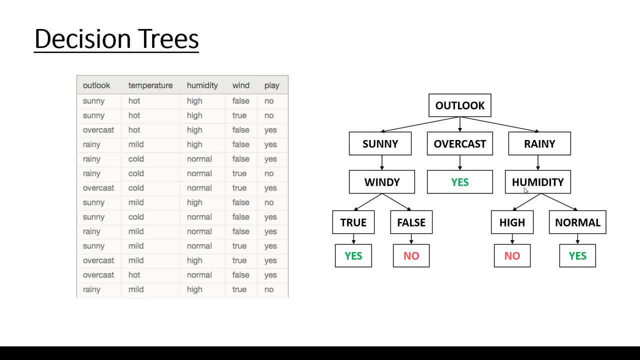 any further. But as far as humidity is concerned, we have to split it into high and normal. As far as wind is concerned, as a feature, we have to split it further into true or false, And the leaf nodes are the target variables, whether we are going to play tennis or not. So, after constructing, 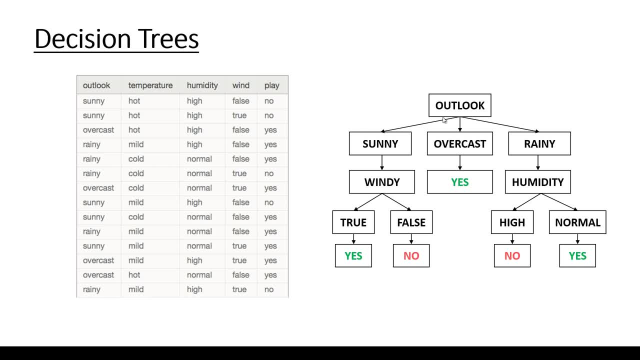 it. we have to split it into high and normal, And we have to split it into true or false, And the leaf nodes are the target variables, whether we are going to play tennis or not. So, after the decision tree based on entropy and information gain, we just have to traverse this tree, like 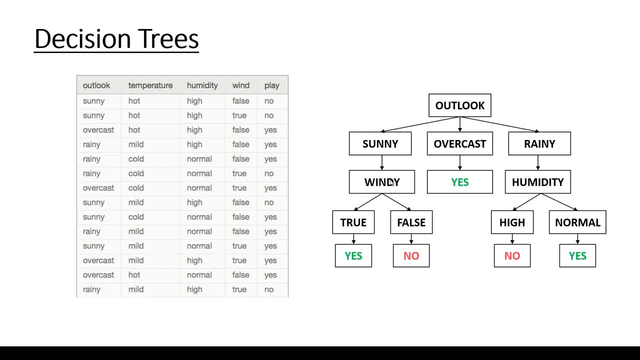 structure. If the outlook is sunny and it is windy, then we are going to play golf. If the outlook is rainy, the humidity is high, we are not going to play golf. So, basically, this is the aim of constructing a tree: like structure, like this, because we are able to predict the target variable. 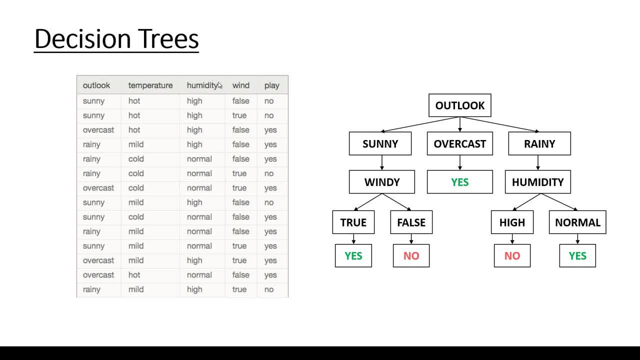 for given features. So if we are going to play golf, we are going to play golf. So if we are going to play golf, we are going to play golf. So if we are going to play golf, we are going to play golf. So 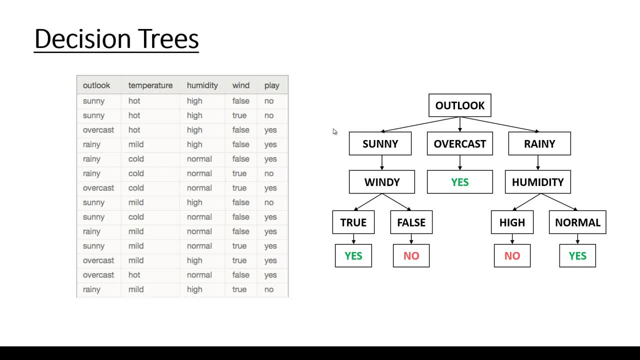 we see the characteristics of a tree as such, as outlook, temperature, humidity and wind. Okay, In the next lecture we are going to talk about the advantages and disadvantages of decision trees And finally, we are going to take a look at the concrete implementation. Thanks for watching. 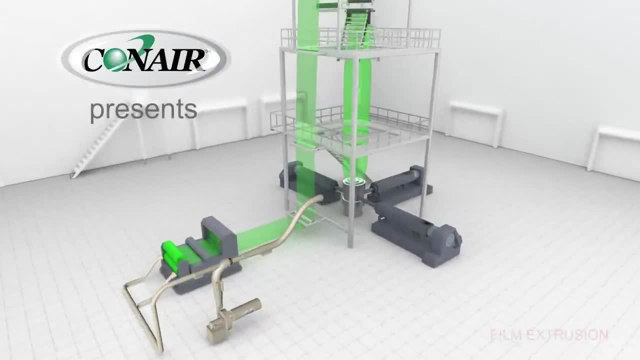 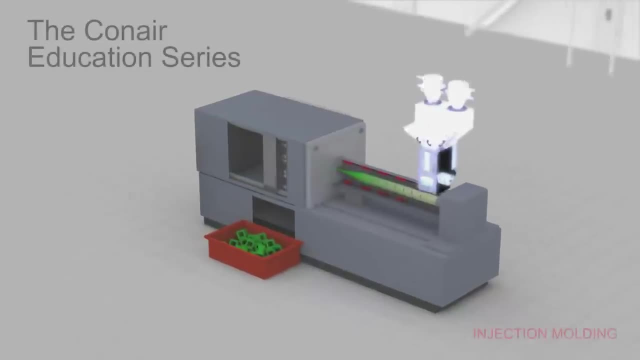 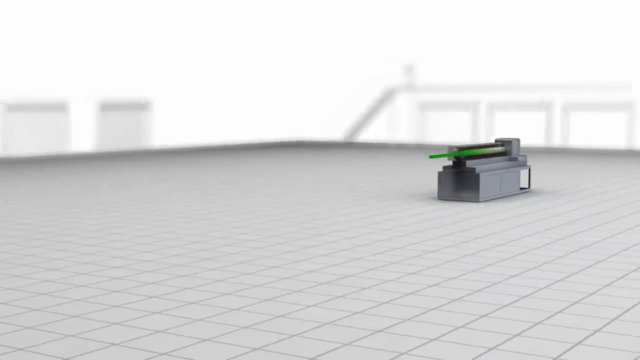 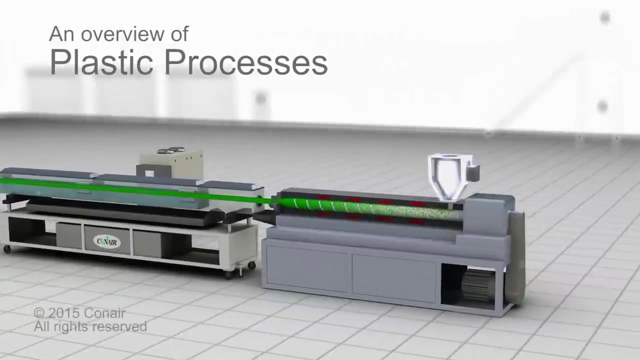 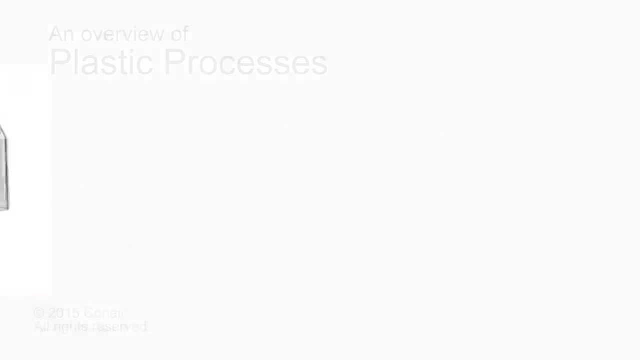 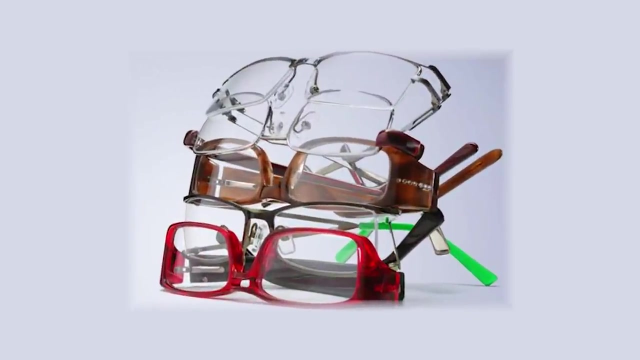 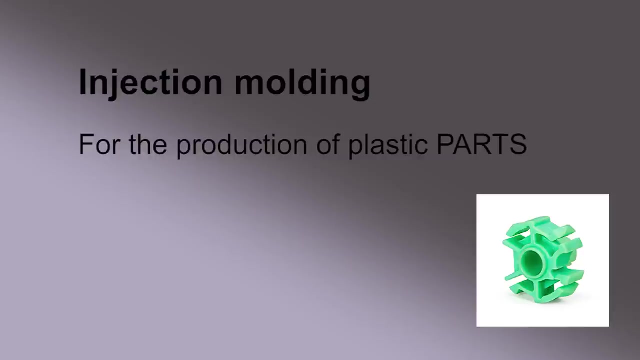 This program will explain the various types of processing machines used to make the wide range of plastic products in use throughout our lives. A good start is injection molding. Injection molding is used to make plastic parts using two-part molds that, when closed, are injected with melted plastic to form. 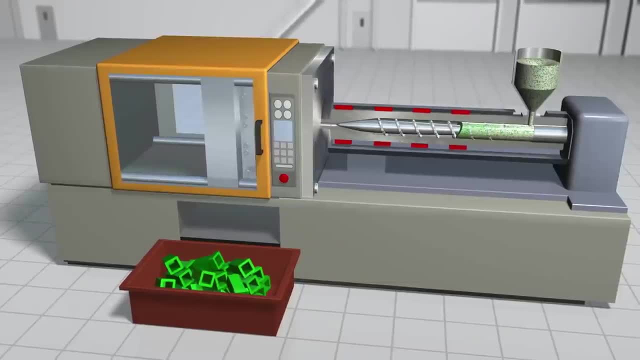 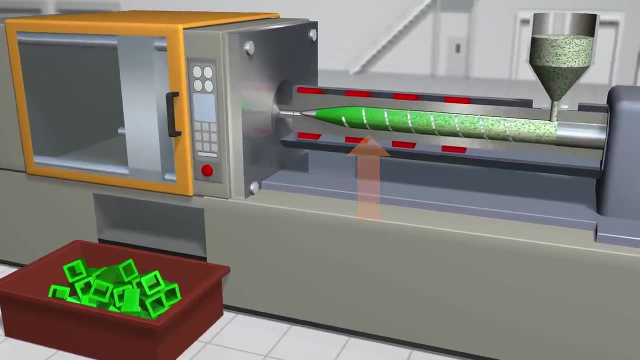 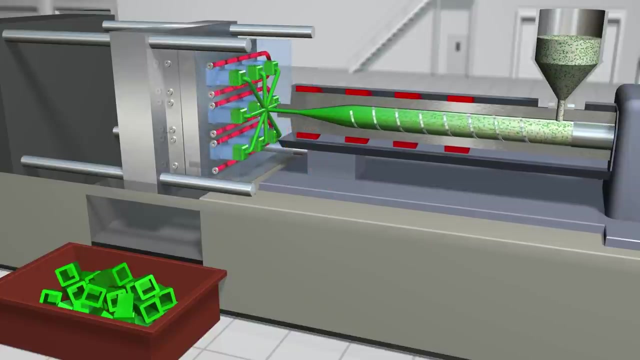 individual parts. Here's how it works: Material gravity flows into the injection machine's screw, where it is melted by the compressing motion of the screw and then injected into the mold to form the part or parts. The mold is quickly cooled, letting the parts solidify. The mold opens to release the